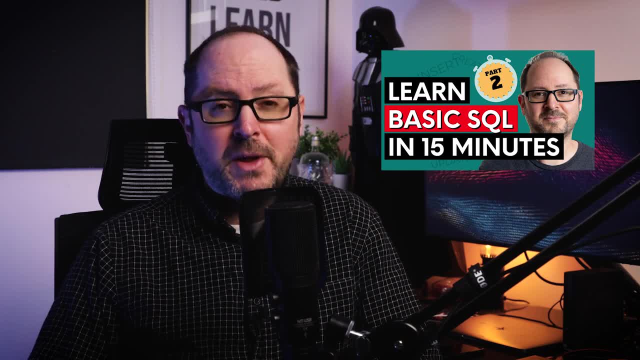 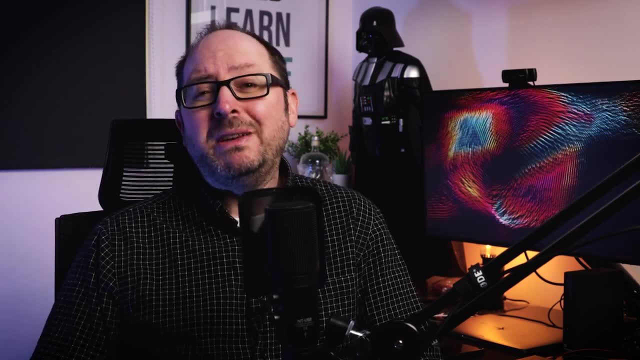 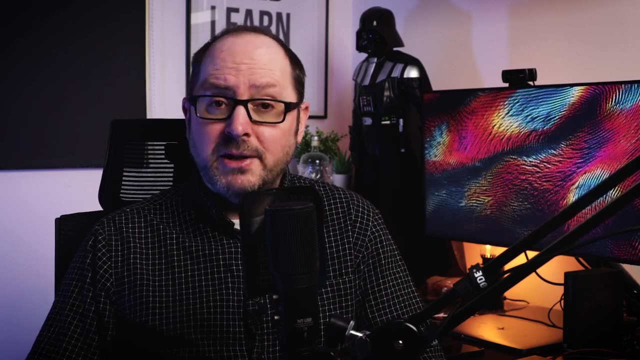 aren't, you might get confused with some of the syntax I use. Okay, let's dive in. So we'll be using a real world scenario, but to keep the whole project more manageable, we'll be simplifying it a little so that these videos don't end up being hours long. Here is the scenario: The client Ben. 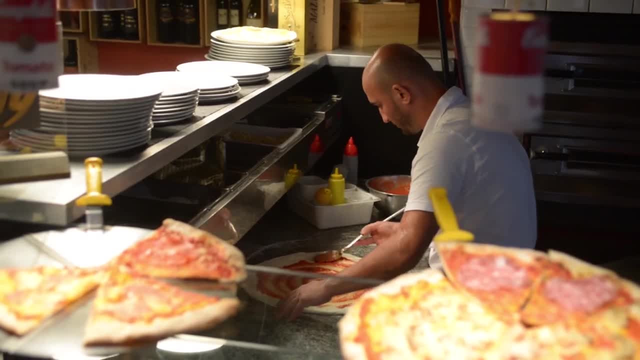 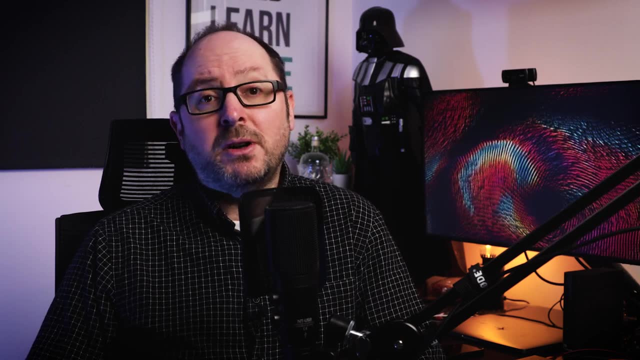 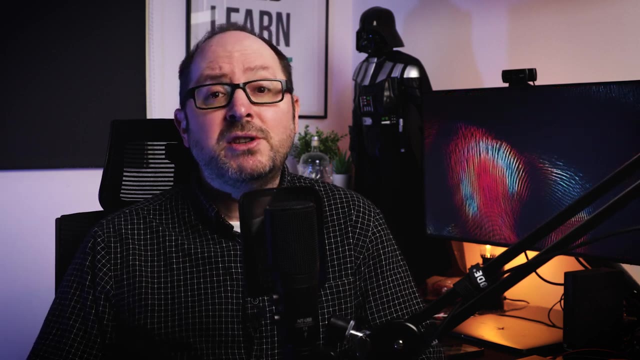 is opening up a new pizzeria in his town. It won't be a day of work, but it's a day of work. He's given us a project brief. The first part requires us to design and build a tailor-made, bespoke relational database for his business that will allow him to capture and store all. 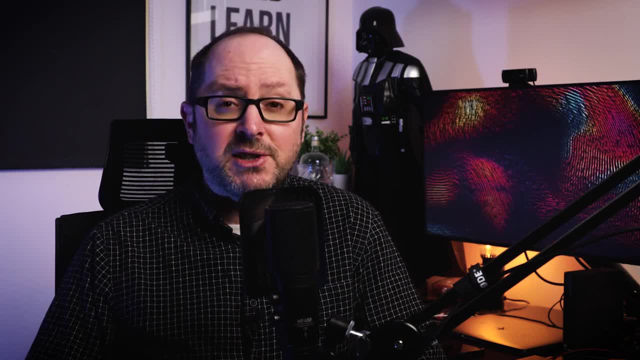 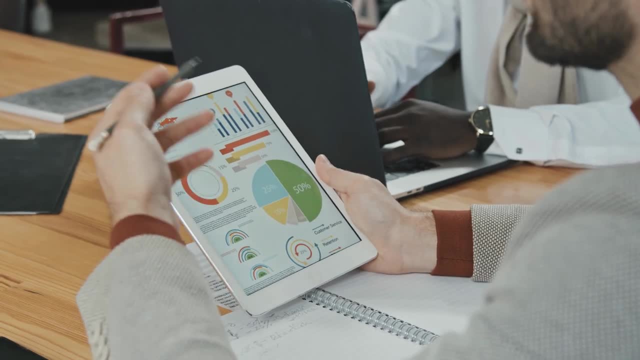 of the important information and data that the business generates. This will, in turn, help Ben to monitor business performance in dashboards that we'll build later on. We're just taking care of the back end. He's hiring someone else to build the front end ordering system. 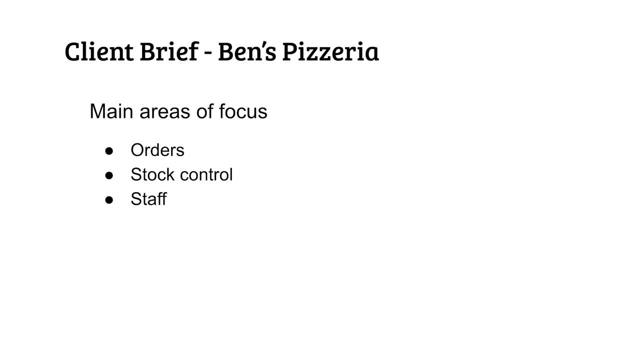 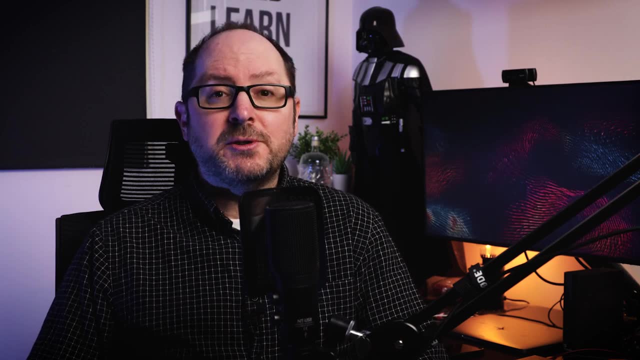 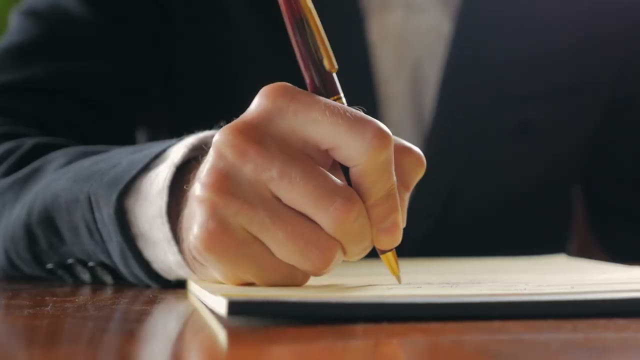 There are three main areas that the brief requires us to concentrate on: Customer orders, stock levels and staff. We're going to start with customer orders. The way we're going to approach this task of designing our database and the tables in it is to spec out all of the fields for the 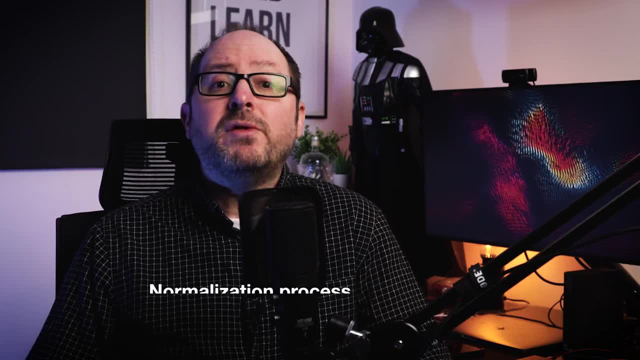 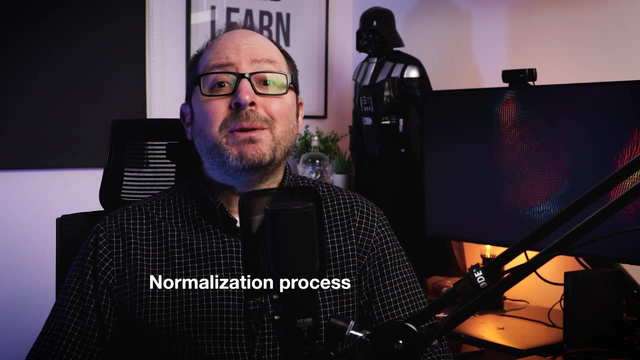 data we want to collect. Then we'll go about the process of normalizing the data, adding more related tables and defining the table relationships. Normalization is something very important in the relational database model and I'll talk more about it in a minute. 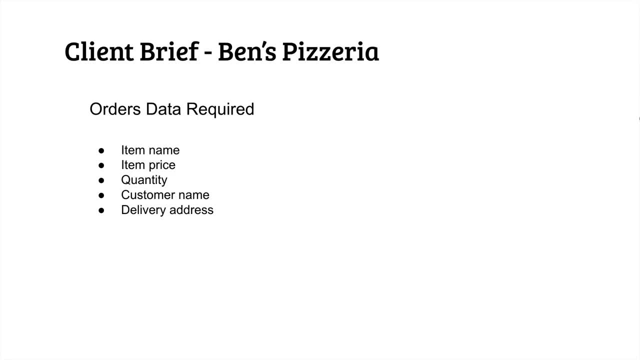 So Ben has given us a list of the different data he'd like to collect for each order. Here it is: Item name, item price, quantity, customer name and delivery address. Now, this list is only the starting point for us to spec out all of the fields we'll need for our orders table. We know 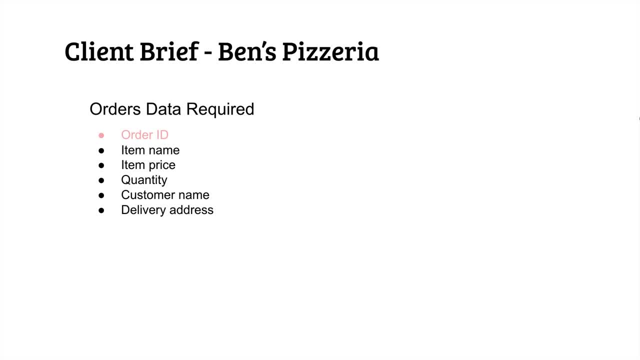 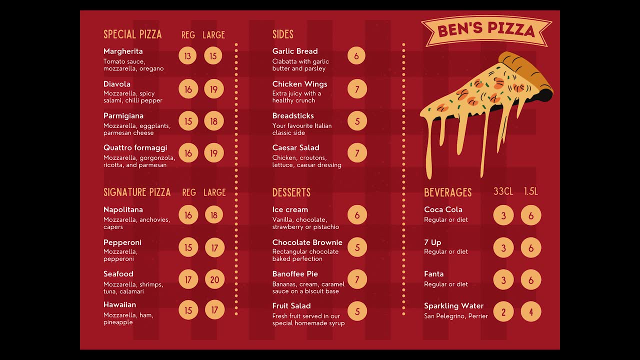 that we're going to need to include things like an order ID field and split out the delivery address parts, And from looking at the menu Ben gave to us, we can see that there are different sizes of pizzas and beverages, so we could include this as a separate field. We could also include a. 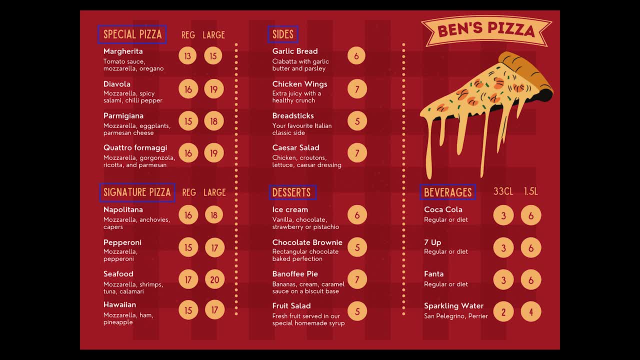 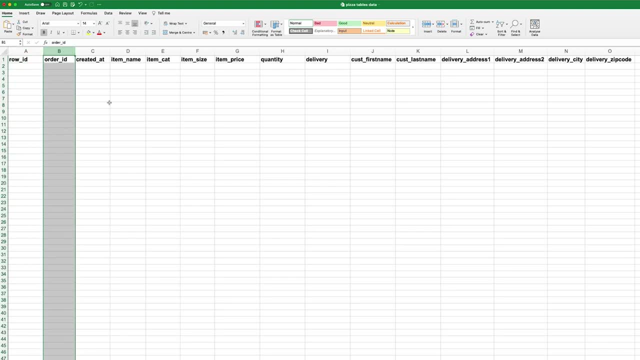 field for the product category. so pizza, sides, desserts and beverages. Here's a mock-up in Excel of what the table could look like. We have our order ID and I've split out the delivery address into different address parts. I've also included a row ID. 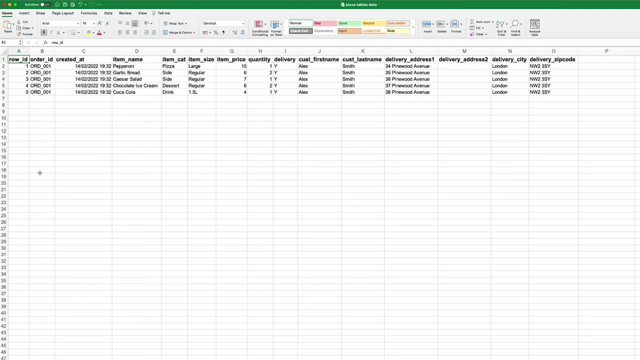 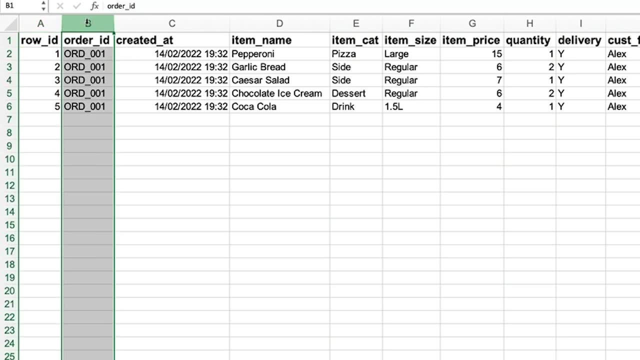 Why did I do this? Well, let's enter data for a first sample order. You notice that each order can contain multiple items. Therefore, we couldn't use it as a primary key to identify each individual row. Hence the row ID that will serve as our primary key. 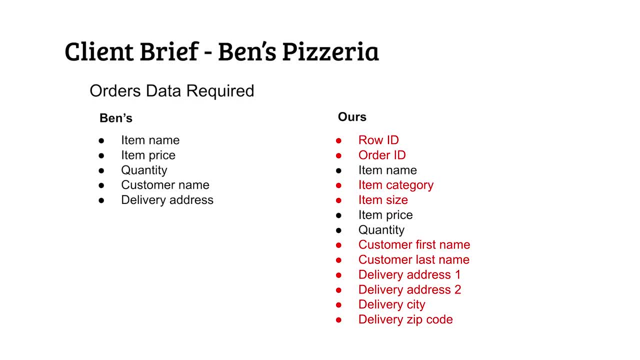 Okay, so now we have an idea of the fields we need for our orders table. I'm going to show you a cool tool we can use to make our job of designing and building our database much easier. It's called Quick Database Diagrams or QuickDBD. 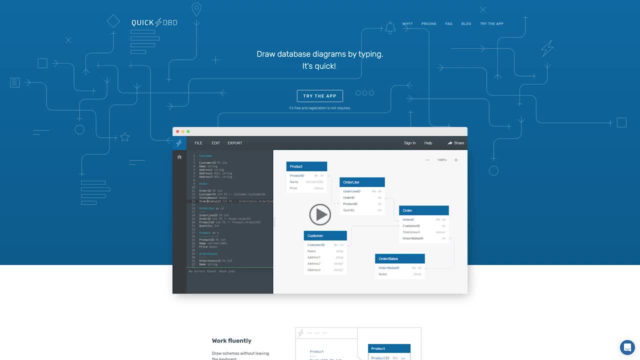 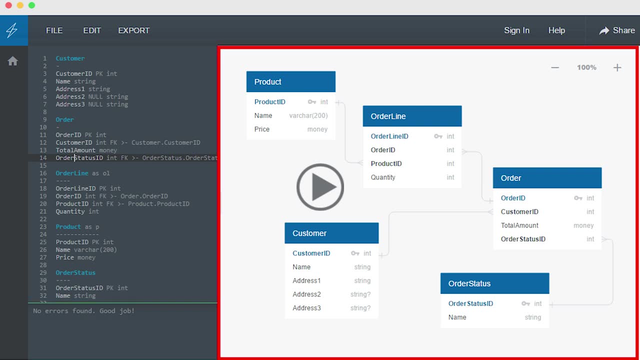 And I'll put a link to it in the description. Basically, you specify here on the left the tables and their fields and on the right. this produces a diagram of our database and its tables. I've gone ahead and created our orders table. 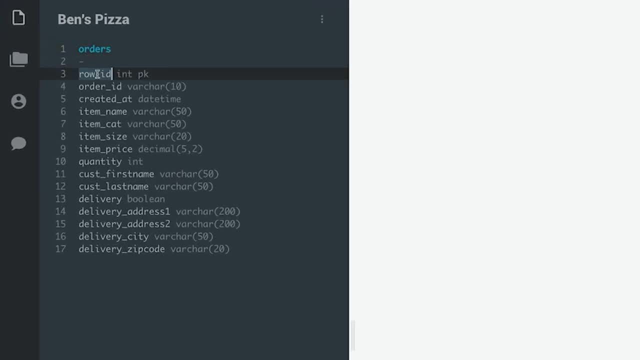 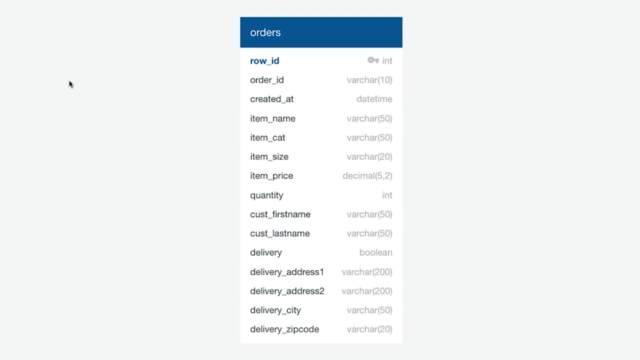 So you can see you need to specify the field name, followed by the data type, And for row ID, I've written PK after the data type to specify it as our primary key. Great, so now we can see what our orders table in its current state would look like. 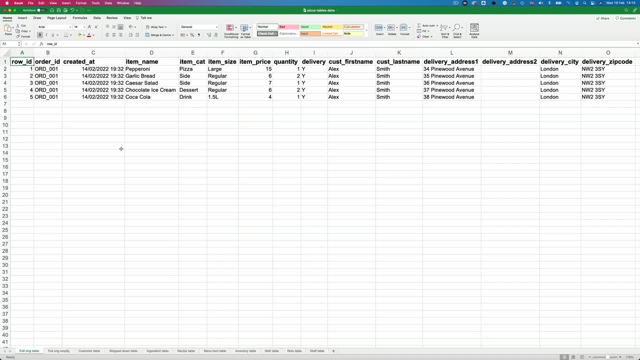 Let's go back to our first dummy order in Excel and take a look at the data. Can you tell me anything that jumps out at you? For me, it's the fact that we have a lot of repetition of data in the various rows. 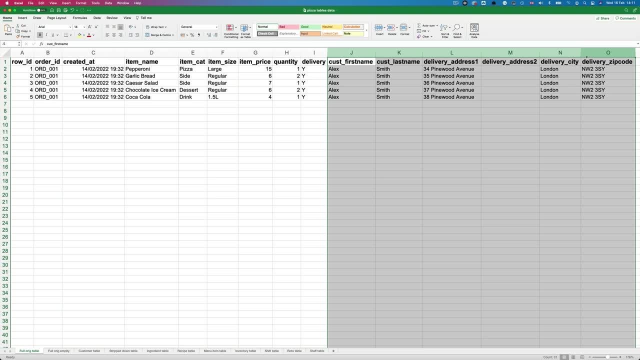 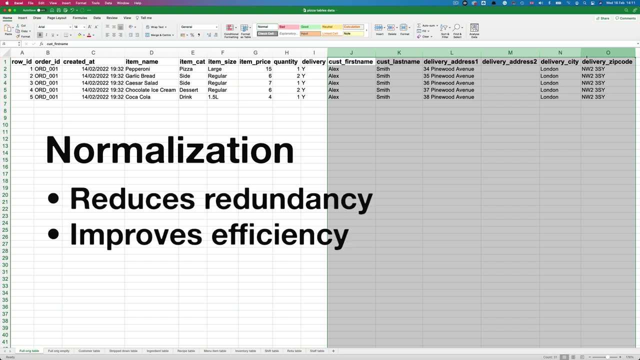 This is called redundancy, and the way we fix it is by what's called normalizing the data. So, essentially, normalizing the data is the process of organizing it to reduce redundancy and make it more flexible and efficient. What we really want to do. 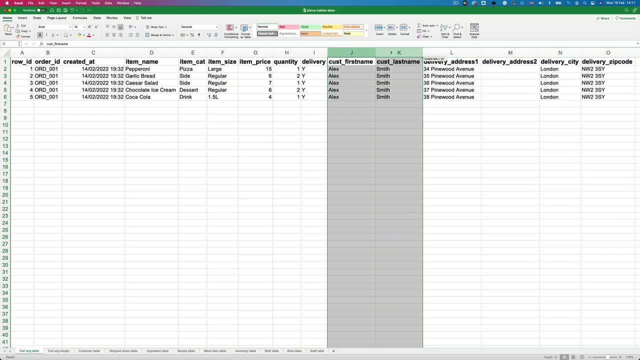 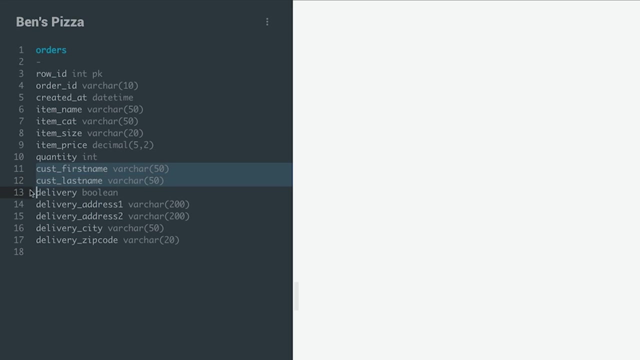 is to create new additional tables for both customers and delivery addresses so that, instead of using all these different fields in the orders data, we can just use and identify it instead. This will, in turn, make the database much more efficient. Let's start with CustomerNames. In the Orders table, we have two fields: FirstName and LastName. 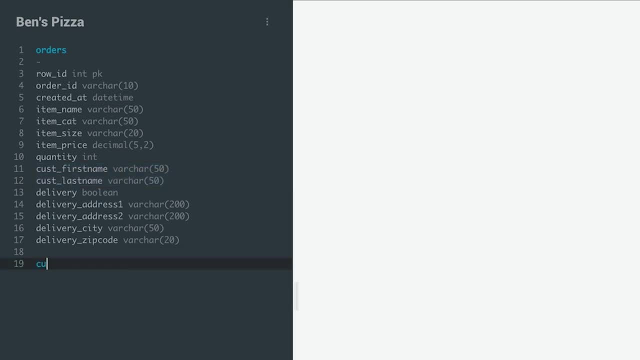 To create a Customer table. here on the left I'm going to write the table name: Customers return- one dash and another return. You'll see that a new table has been added to the diagram In this Customer table. I'm going to start by adding CUST underscore ID with: 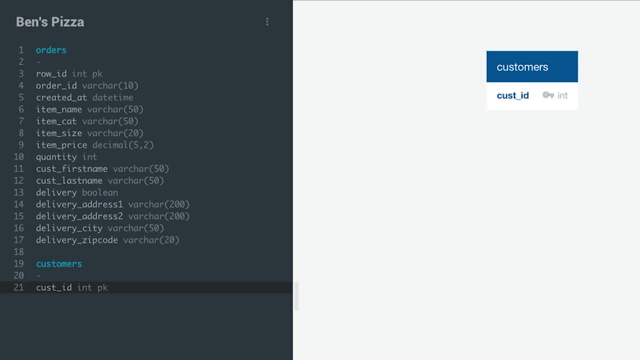 an INT datatype as a primary key, Then I'm going to cut the two Customer field names from the Orders table and paste them into our new Customers table. That's great, but now we need to replace those two fields in the Orders table with the Customer ID field. 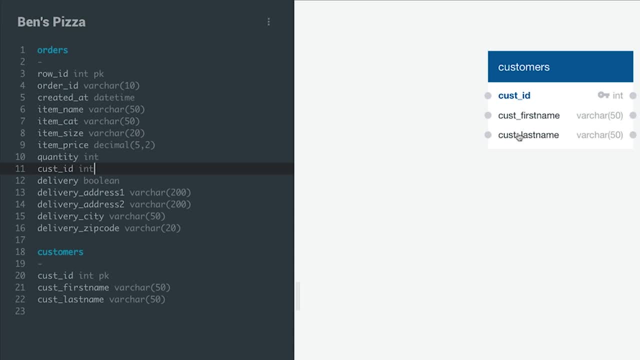 as an identifier, Like so. Now, all we need to do is to specify the real name of the customer. Now, all we need to do is to specify the real name of the customer. Now, all we need to know is, we need to know the relationship between these two tables. I do this by dragging. 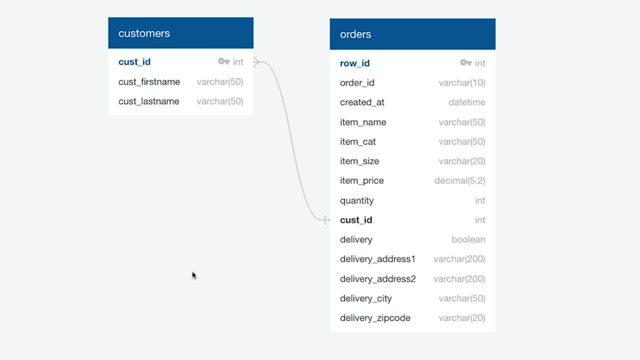 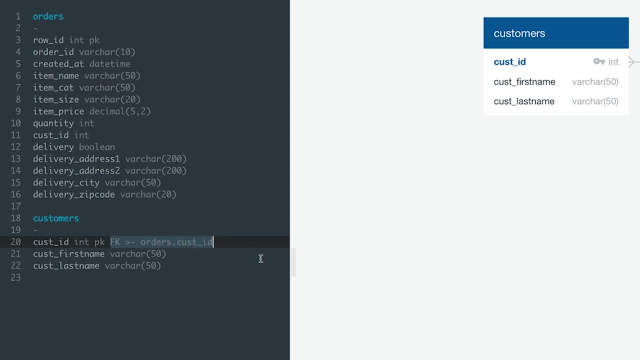 from CUST ID in one table to CUST ID in the other. In our syntax on the left we can see that CUST ID has now been specified as a foreign key connected to ordersCUSTID. Make sense? There are some slight differences here. let's continue. 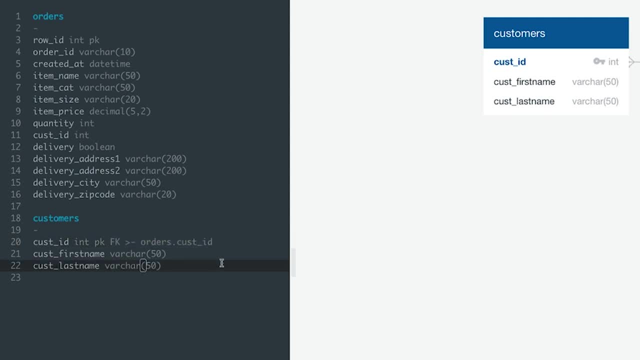 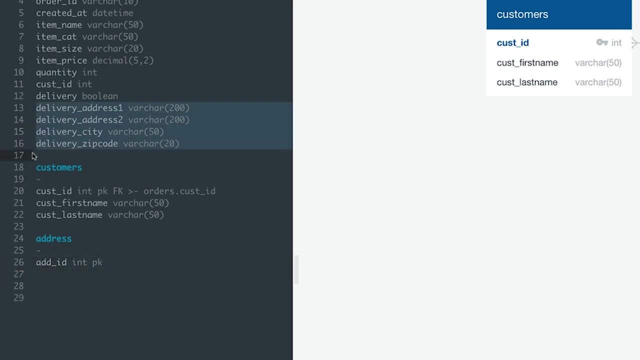 Let's do a similar operation for our delivery addresses. I'll create a new address table containing an Address ID, just like in the moment. We will cut the address fields from orders table and paste them into the address table and make sure to add the address ID field to the orders table in their place. there's one more thing. we 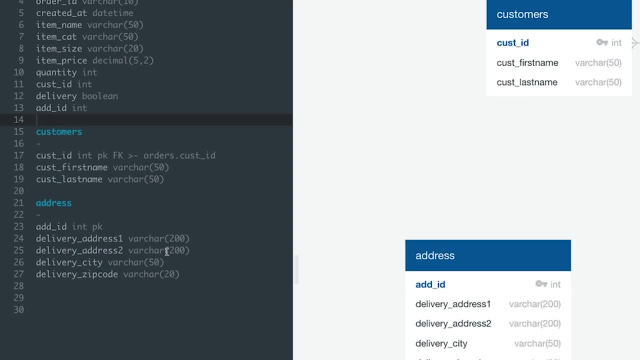 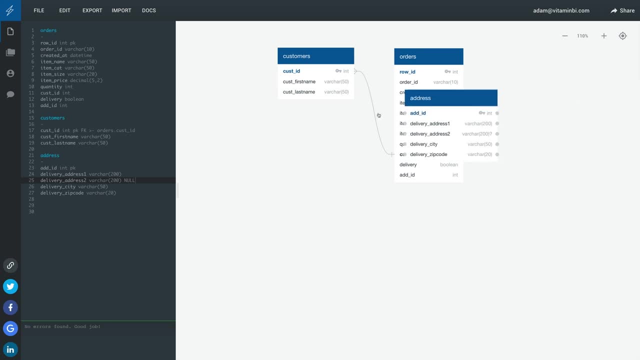 need to do to the address table, and that is to add a null constraint to the delivery underscore address to field. the reason for this is that, by default, quick dbd applies the not null constraint to every single field, meaning that it cannot contain null values. however, the delivery underscore address to field is: 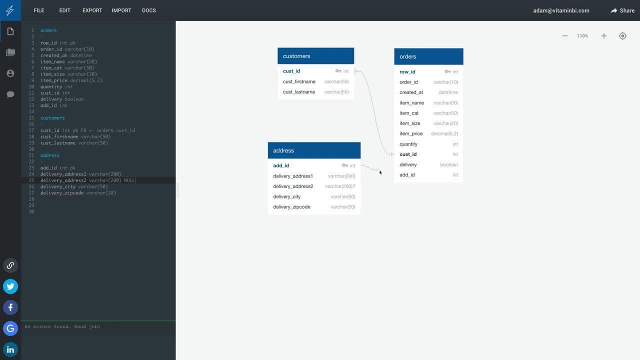 not always needed, so can, in fact, be null. once that's done, I will then specify the relationship between the address and orders tables. now this is looking a lot better, but I'm also going to need to create a product or item table. this will serve two main purposes. first, it will reduce the amount of data in the table. 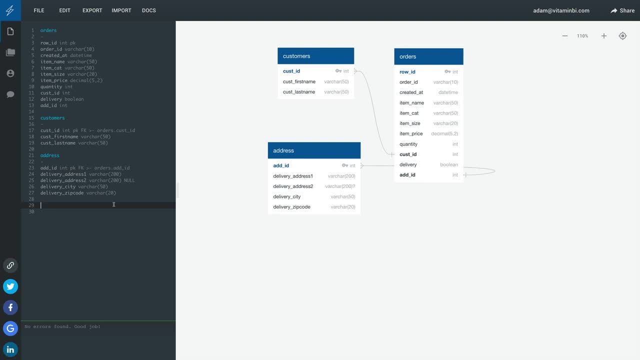 like with the other two examples, and then I will specify the relationship between the address and orders table. and second, let's imagine that at some point Ben might want to change the name of an item. if we have an item table containing a list of all menu items, we would only 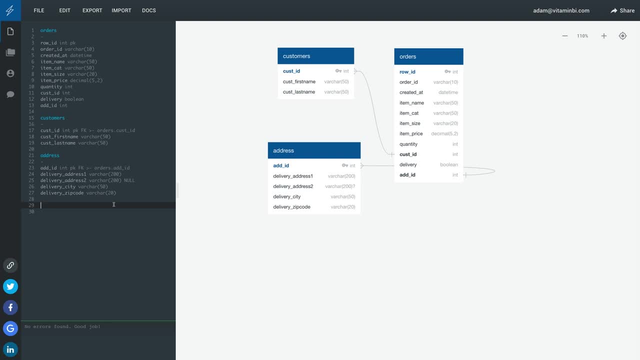 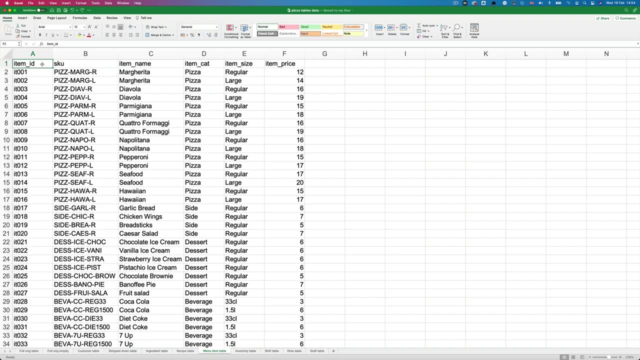 need to change one row of data in the table rather than changing all the rows in the orders table where the item existed, much more efficient. here in Excel, I have what the item table data looks like. we have item ID, skew, item name, item category, item size and item type. 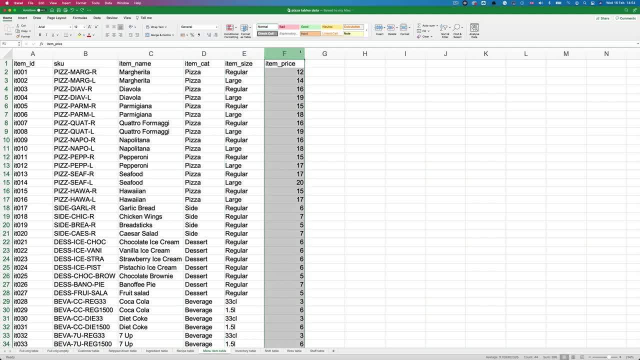 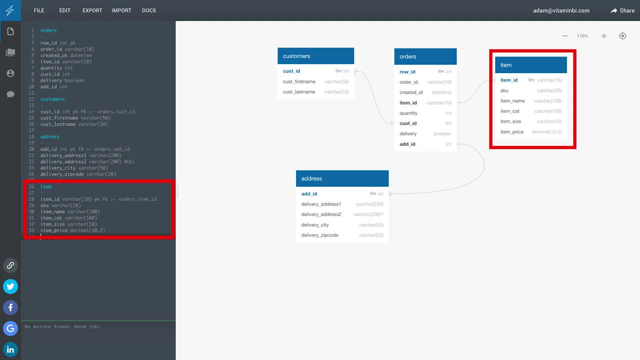 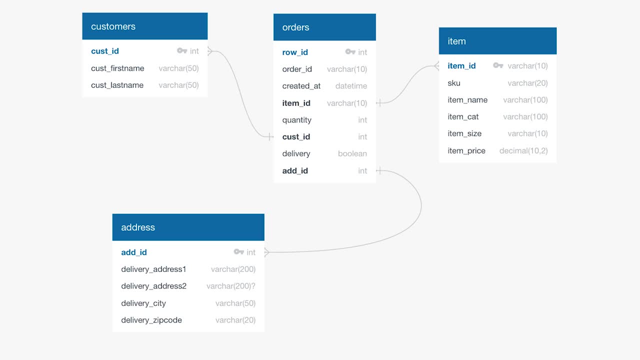 and item price. I'm going to go ahead and create this new item table and specify the relationship in Quick DVD like so: looking good, and that is the orders part taking care of. next up, we're going to start thinking about the stock control part that Ben wants us to include, but before we do, I just like to 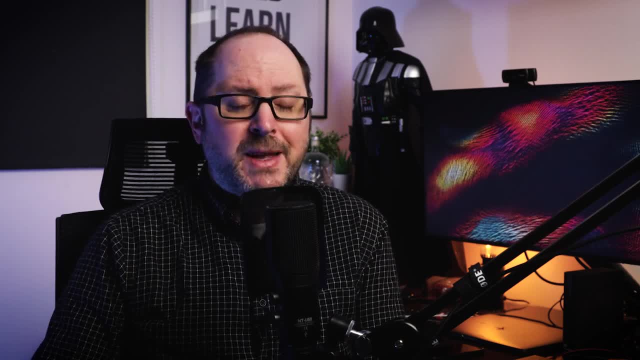 say that if you're intending to follow along with this project all the way through, I'm going to need your help. essentially, I can only build and easily populate certain photos and wide fields at the same time, and a simple success will certainly work to produce creating the evidence about the focus, internal JSONろing for an item, as well as the data. 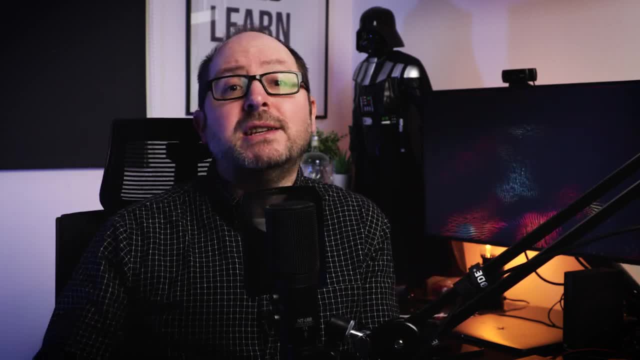 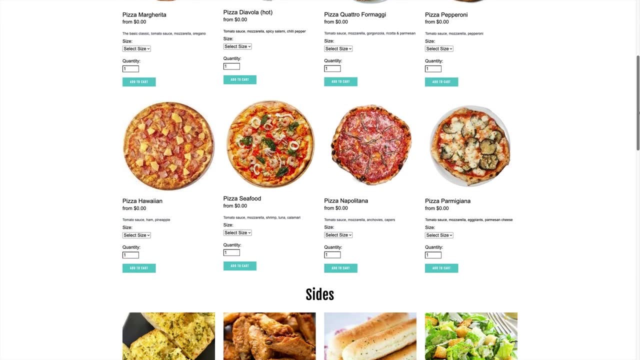 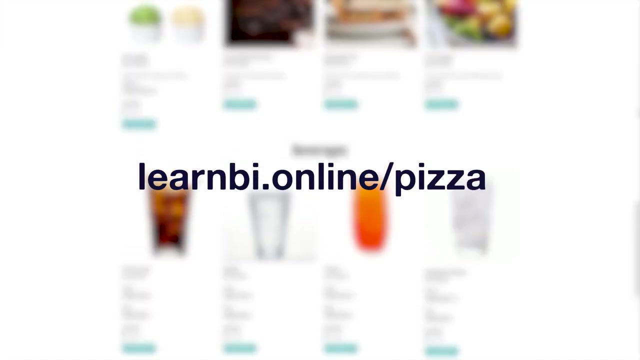 tables. but in order to generate some real data for the orders tables, I've set up an online ordering page. it's got the full menu and will allow you to place as many orders as you like, which will then be used to populate the orders tables. just go to learn bi dot online slash pizza, or click the link in the 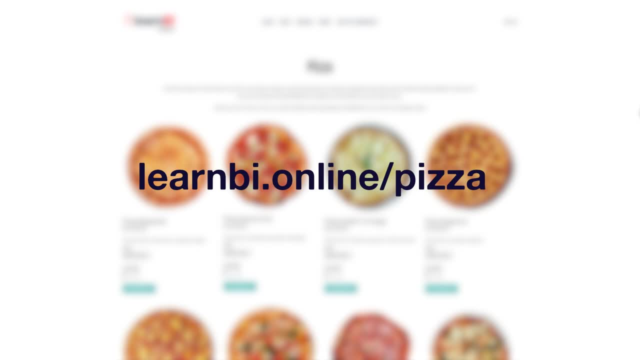 description after this video and place an order. if you do, you'll be able to get your hands on a copy of all the data once it's been collected, as well as the finished sequel code for creating the database. you'll find the full instructions also in the description below. for now, keep watching and I'll 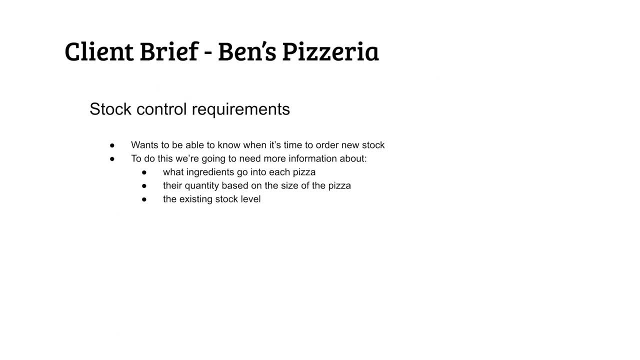 remind you again at the end of the video. so for the stock control data, essentially, what Ben would like to be able to do is to put in place a way for him to know when it's time to order new stock. to do this, we're going to need 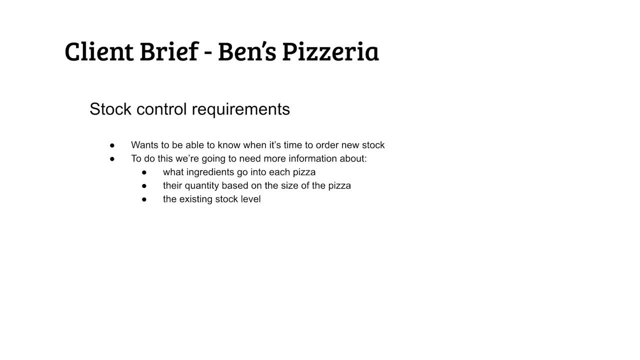 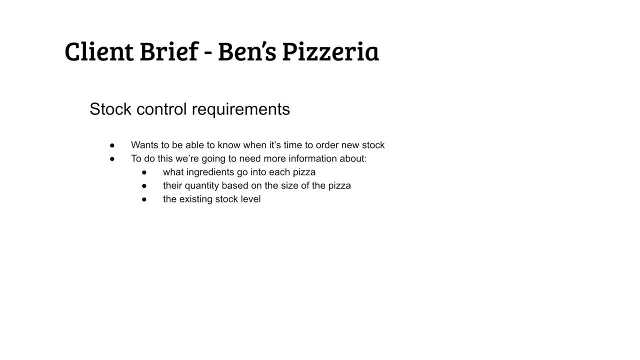 different suppliers in delivering new stock, which would mean as needing to calculate exactly when to reorder each item or ingredient. but I think, to keep things more simple, we'll just assume that the lead time for all items is the same, so Ben has kindly supplied us with the necessary information on each pizza. 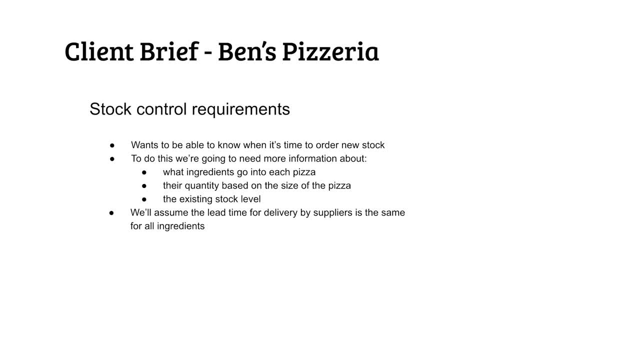 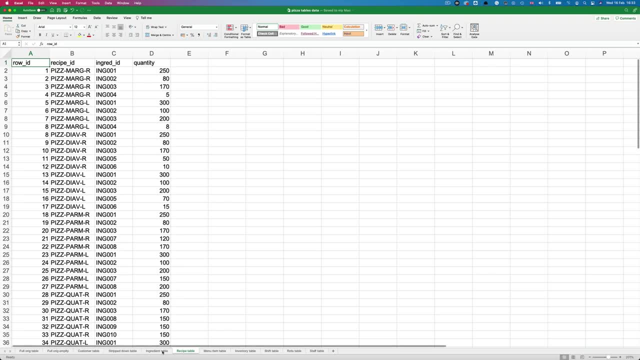 and the weight that the item is sold in. he's also given us a list of the ingredients and the amounts that go into each pizza. I've turned all of this information into two separate tables that I'm going to create in quick DVD. we can see from the data that the recipe ID is the same as the SKU from the item. 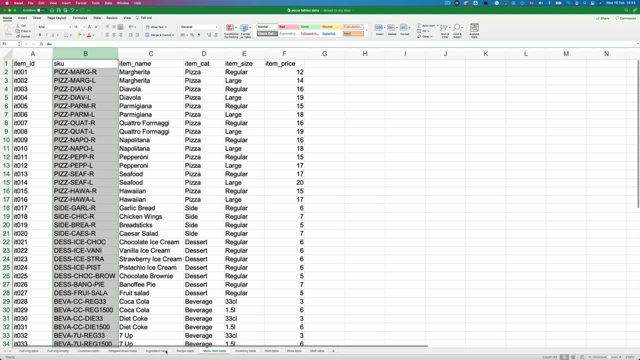 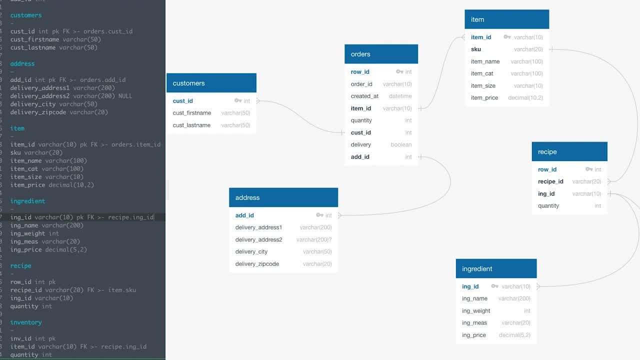 table and the ingredient ID appears in both the ingredient and recipe tables. so those are the relationships that I've specified. with all of this data, Ben's will be able to calculate exactly how much each pizza costs to make. if supplier prices go up, he'll just need to update the ingredient prices in the ingredients. 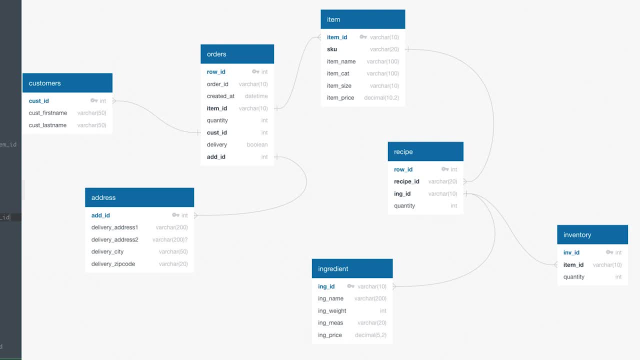 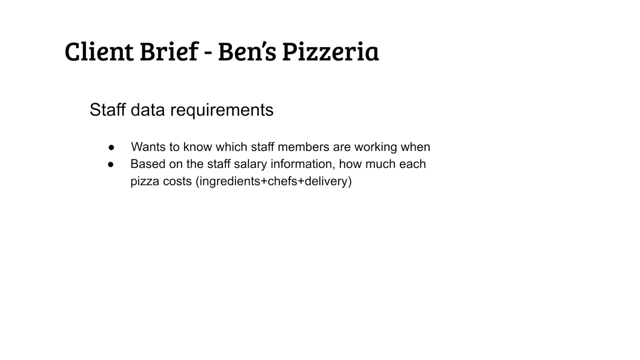 table. finally, we'll need a table to hold stock levels for each ingredient. this inventory table will contain inventory ID, item ID and quantity fields. and that's it for the stock control part. the final part is staff data. according to the brief, Ben would like to know two things: which staff members are working when, then, based on their salary? 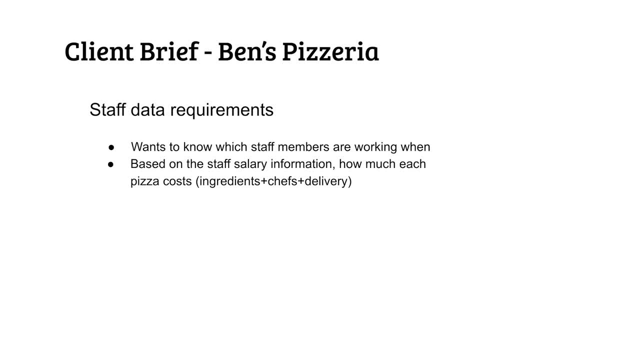 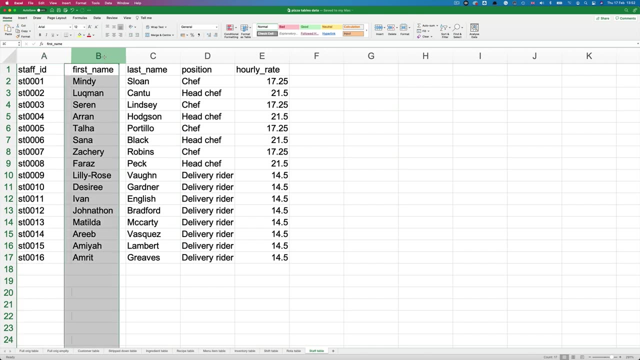 information how much each pizza is actually costing him, not only in terms of ingredients, but also the chefs making the pizza and the cost of delivery based on the time it took to deliver. let's start with the staff table. here it is in Excel. we have staff ID, staff first name, staff last name, position and hourly rate. 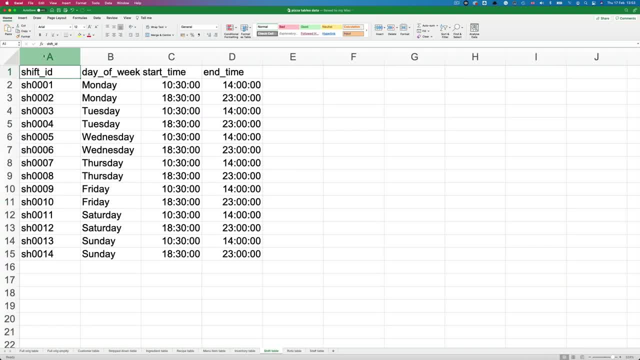 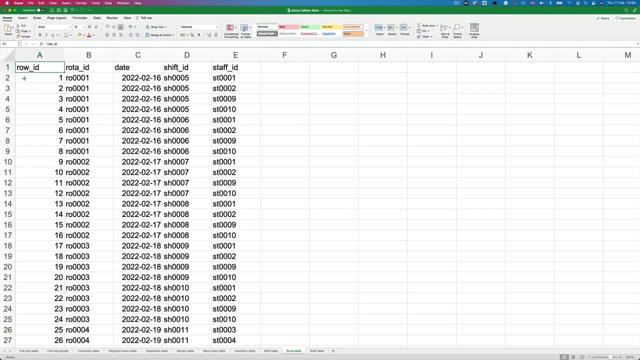 then we have a shift table. this contains shift ID, the day of the week, the start time and finish time. most staff work both the lunch time and evening shifts on any given day, but some do not, which is why we need to split them up. the final table we're going to need is the rotor table. this will tell us who is working. 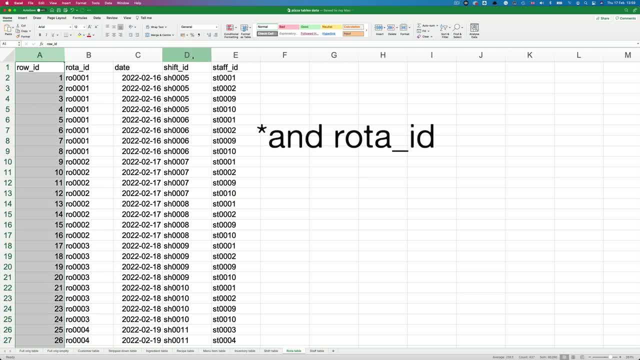 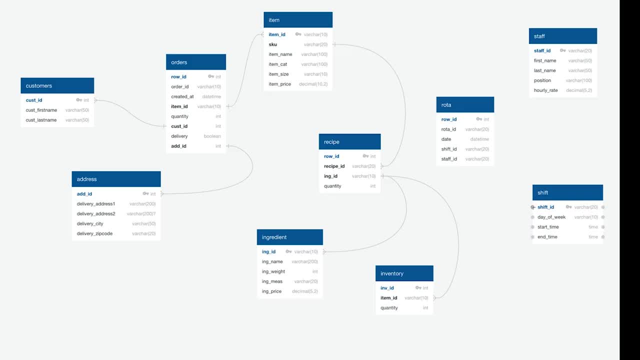 when for this we'll need a row ID, a shift ID, the date and the staff ID. the relationships between the three tables are: shift ID from the shift table to shift ID in the rotor table, then staff ID from the staff table to staff ID in the rotor table and finally, date from the rotor table to created. 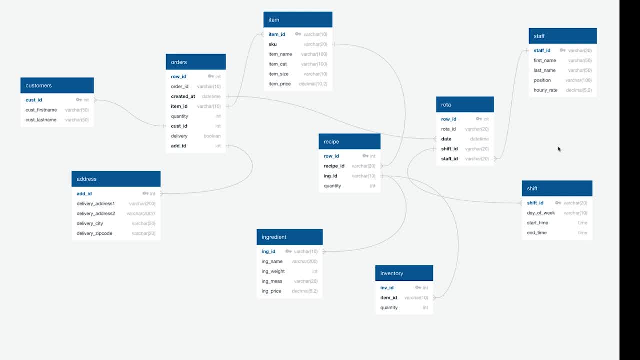 date in the orders table. this last one will give us the join we need between the staff tables and the order tables. now we have everything we need for Ben's database, at least for this simplified scenario. once we've designed the database, there's just the small matter of creating it to be done. fortunately, this is where quick dbd makes life very easy. 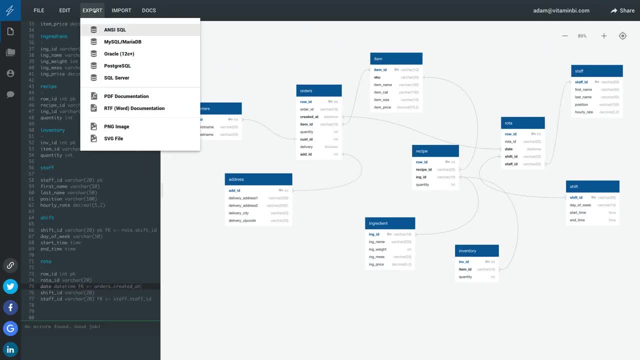 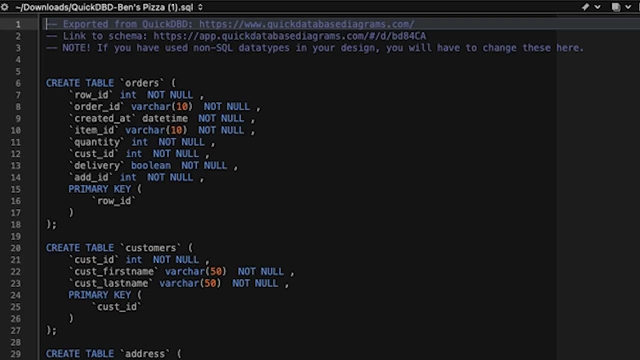 indeed, all I need to do is to go to the export menu, where I can choose to export the SQL code into a variety of different rdbms syntax. I'm going to be using my sequel, so I'll select this option. if I open the downloaded file, you can see that it contains all the code needed to create the tables. 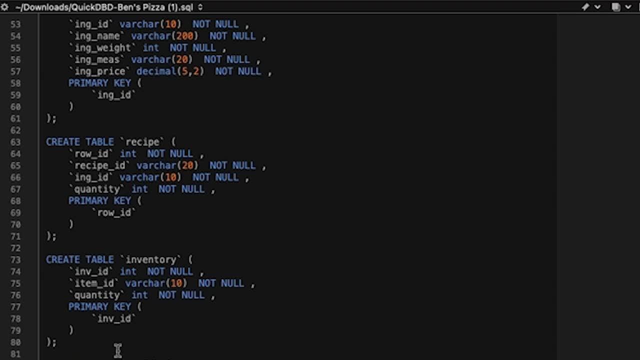 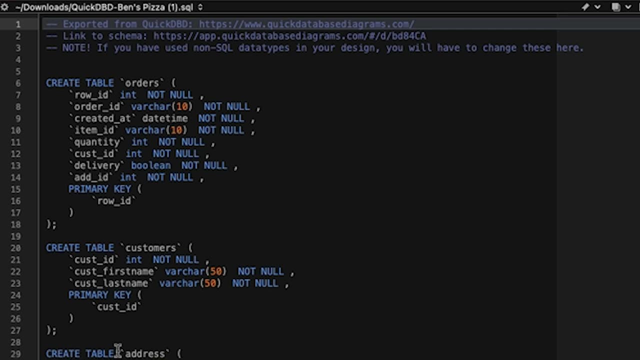 so at this point you might be thinking: but how do I get access to an instance of my sequel? well, it's actually not that difficult. I'm not going to go into it in this video, maybe I will in another one, but just search on YouTube for how do I install my sequel on my computer? once it's installed, you'll be able to create. 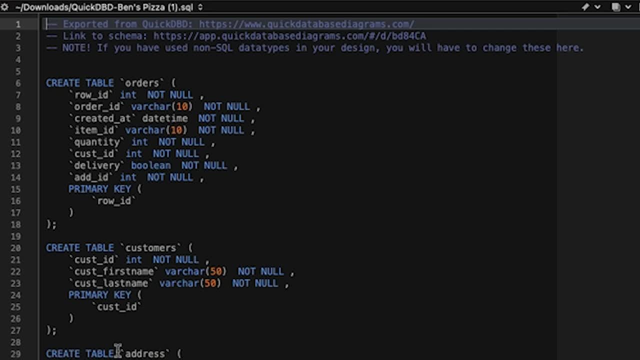 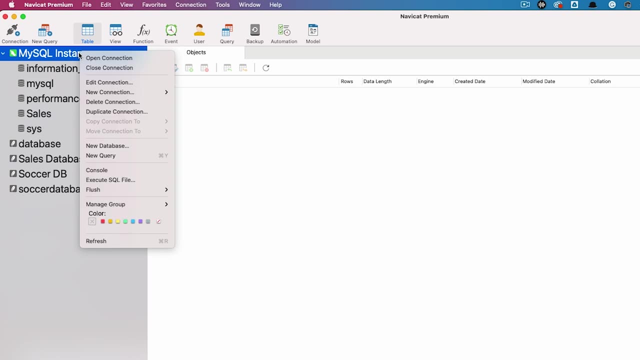 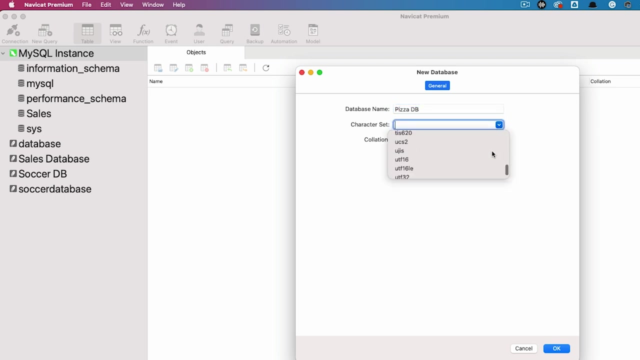 connections to it so that you can then create databases, like I'll be doing now in NaviCat- link in the description. if I go into NaviCat I can right click on my my SQL connection and create a database. I'll call it pizza DB. for the character set I'll choose utf-8, mb4 and I'll set collation to. 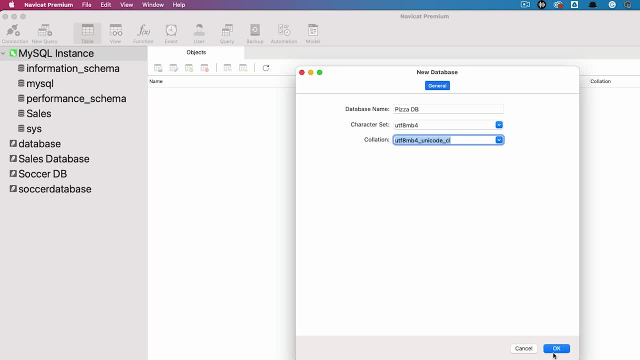 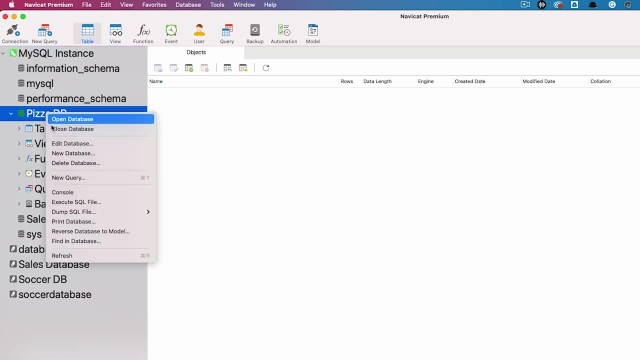 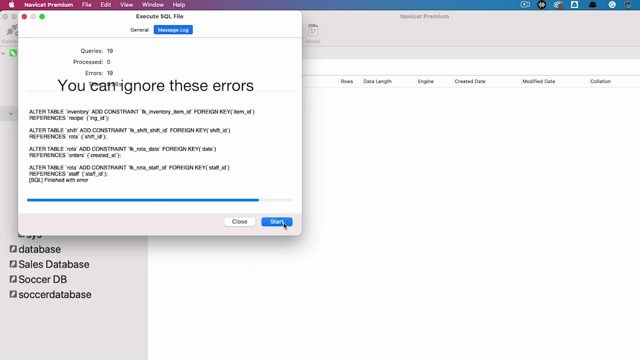 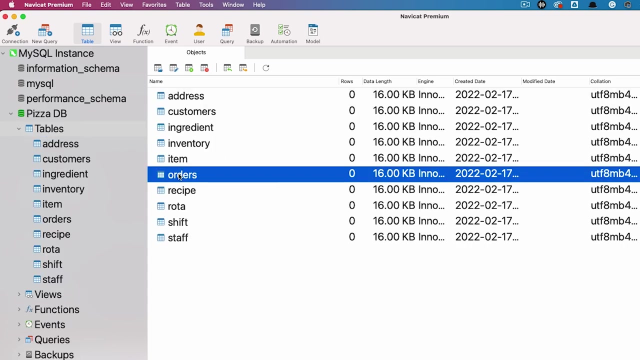 utf-8, mb4, underscore, Unicode, underscore CI. and here it is on the left to create our tables in this database. I'll right click and select execute SQL file. choose my SQL file and run. hey presto, the tables have now been created in my database. I can now populate the tables. 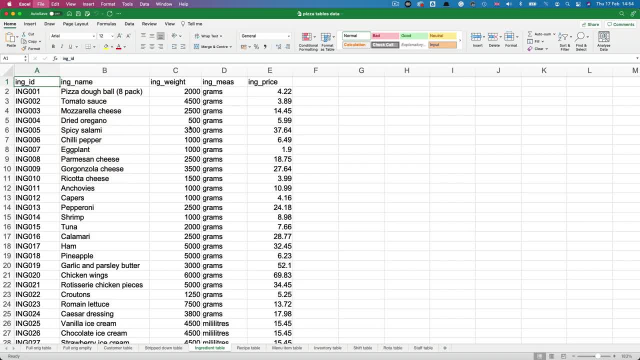 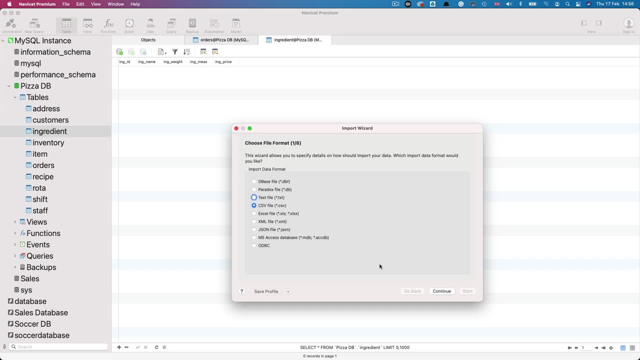 where I already have the data. I've downloaded the ingredients Excel sheet as a CSV file and now I can just use the NaviCat import wizard, select CSV, add the file, continue, continue, continue. the target table is ingredient. check the fields are correct and then either use the append.